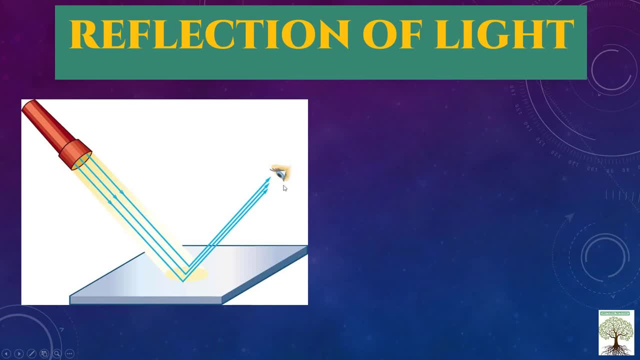 Then this opaque object reflect this light in our eyes or bounce back the light in our eyes so that we are able to see this opaque object. Okay, So this is the property of light: Reflection of light. When light falls on an object, opaque object, this object will bounce back or reflect back this light in our eyes so that we can see the opaque object. 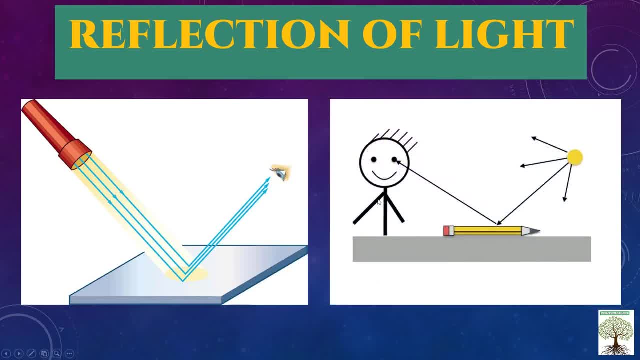 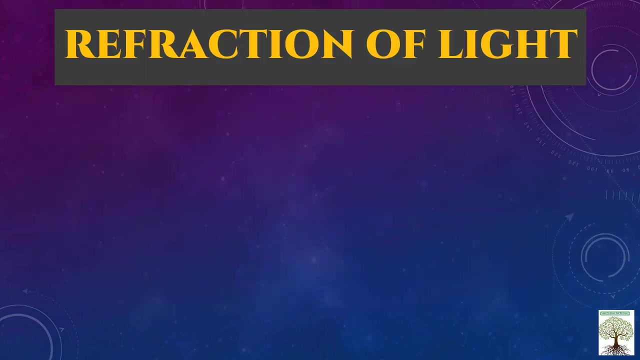 This is the property of light. In this picture we can see that sunlight is falling on this pencil and pencil reflect back this light, sunlight in the eyes so that we can see the pencil. We are able to see the pencil. This is the property of light. Reflection of light. Next property: refraction of light. Here, as you can see, when light travels in a straight line, light travels in a straight line. This is the property of light. 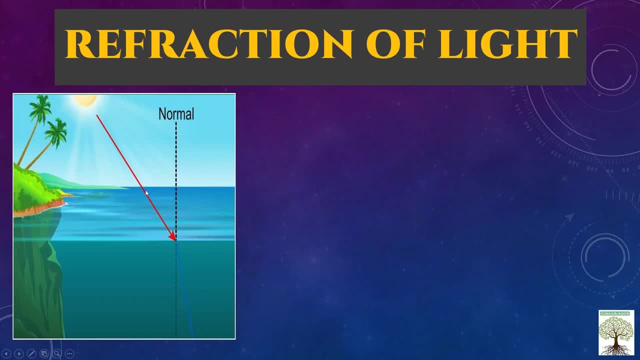 When light travels from one medium to another, that means when light travels from air to water or any other medium, this light bends over the boundary here, at the edge. So light bends at the edge, at the boundary. This is the property of light. Refraction of light. When light pass from one medium to another, from air to water, it will bend It little bit, bend. Light bends at the boundary. This is the property of light. Refraction of light. When light pass from one medium to another, from air to water, it will bend It little bit, bend. Light bends at the boundary. This is the property of light. Refraction of light. When light pass from one medium to another, from air to water, it will bend It little bit, bend. Light bends at the boundary. This is the property of light. Refraction of light. When light pass from one medium to another, from air to water, it will bend It little bit, bend. Light bends at the boundary. This is the property of light. Refraction of light. 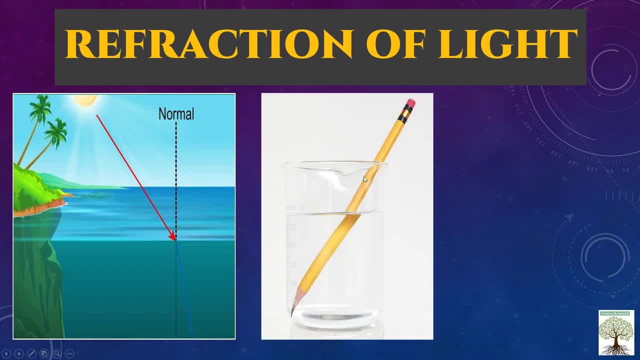 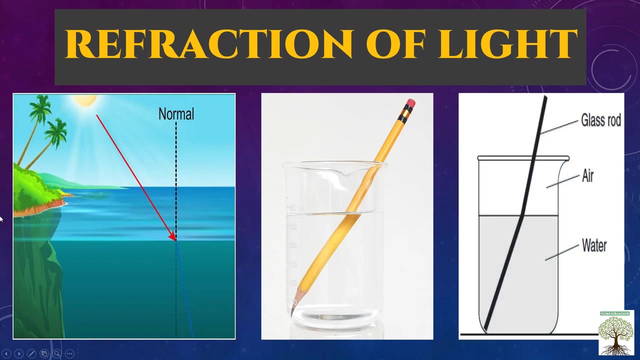 this is the property of light. see the pencil. due to refraction of light we are able to see pencil like this. ok, so light travels from one medium air to water, so it will bend, little bit bend, so this is known as refraction of light. as you can see here, glass rod is. 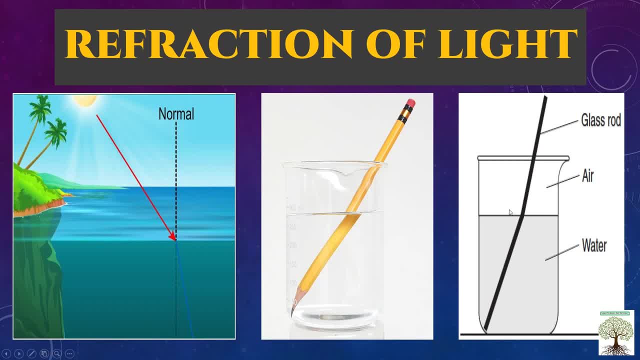 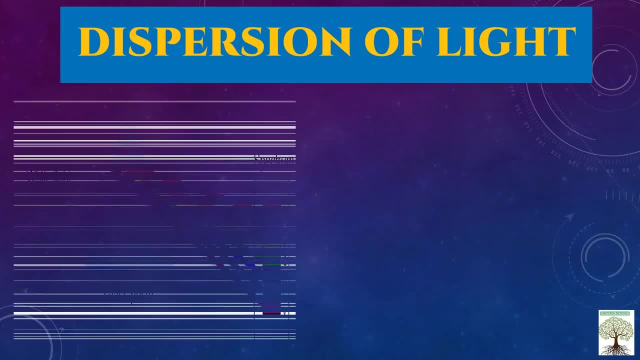 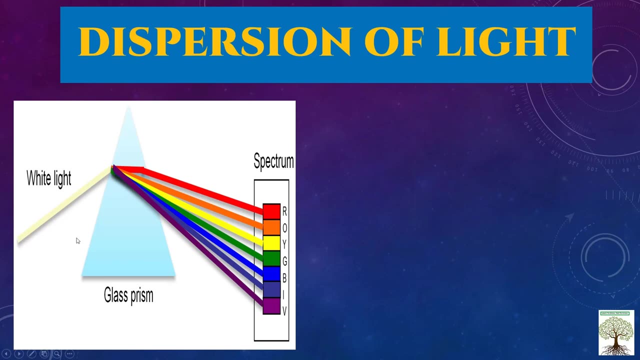 there, air to water. this is bend, little bit bend. so this is the refraction of light. next property is dispersion of light. what is dispersion? the white light of the Sun is actually made up of the seven colors. not only Sun, any white light is made up of seven. 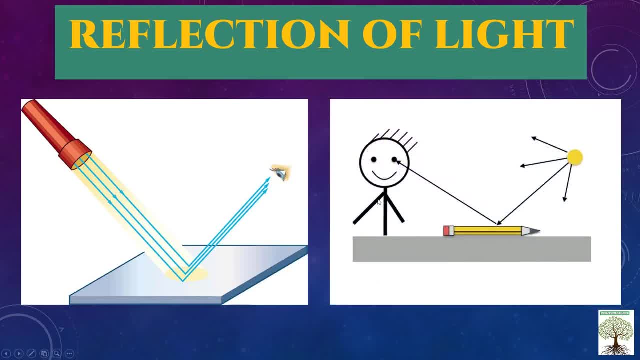 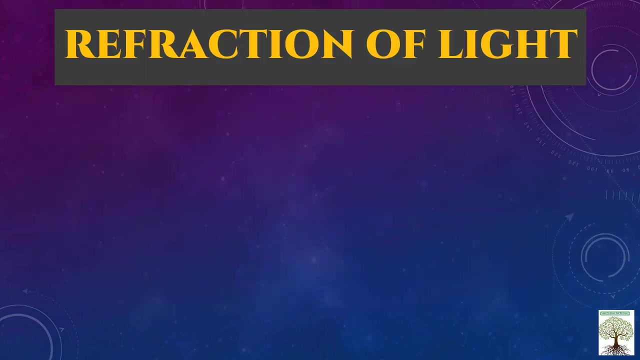 This is the property of light. In this picture we can see that sunlight is falling on this pencil and pencil reflect back this light, sunlight in the eyes so that we can see the pencil. We are able to see the pencil. This is the property of light. Reflection of light. Next property: refraction of light. Here, as you can see, when light travels in a straight line, light travels in a straight line. This is the property of light. 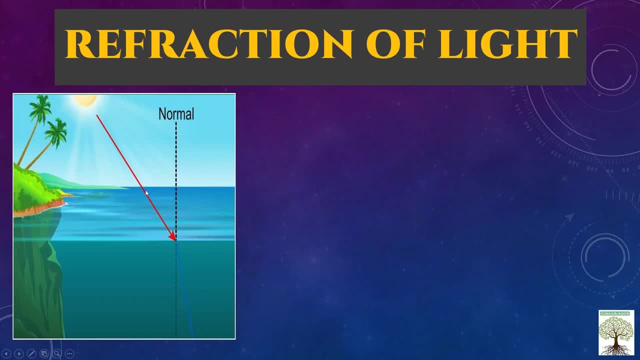 When light travels from one medium to another, that means when light travels from air to water or any other medium, this light bends over the boundary here, at the edge. So light bends at the edge, at the boundary. This is the property of light. Refraction of light. When light pass from one medium to another, from air to water, it will bend It little bit, bend. Light bends at the boundary. This is the property of light. Refraction of light. When light pass from one medium to another, from air to water, it will bend It little bit, bend. Light bends at the boundary. This is the property of light. Refraction of light. When light pass from one medium to another, from air to water, it will bend It little bit, bend. Light bends at the boundary. This is the property of light. Refraction of light. When light pass from one medium to another, from air to water, it will bend It little bit, bend. Light bends at the boundary. This is the property of light. Refraction of light. 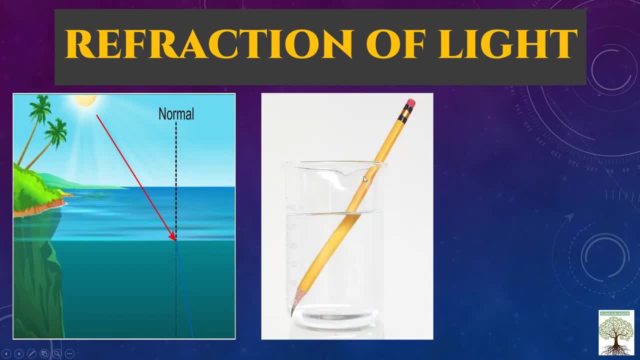 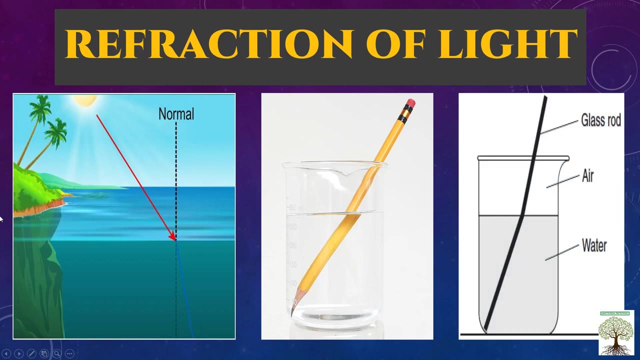 When light pass from one medium to another, from air to water, it will bend It little bit bend. Light bends at the boundary. This is the property of light. See the pencil. Due to refraction of light, we are able to see pencil like this. Okay, So light travels from one medium- air to water, So it will bend, Little bit bend. So this is known as refraction of light. As you can see here, glass rod is there. Air to water- This is bend, Little bit bend. So this is the refraction of light. 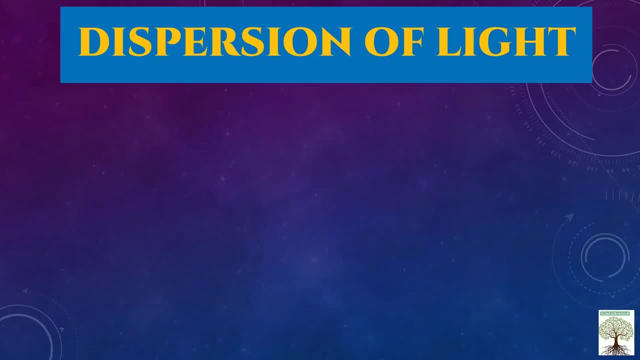 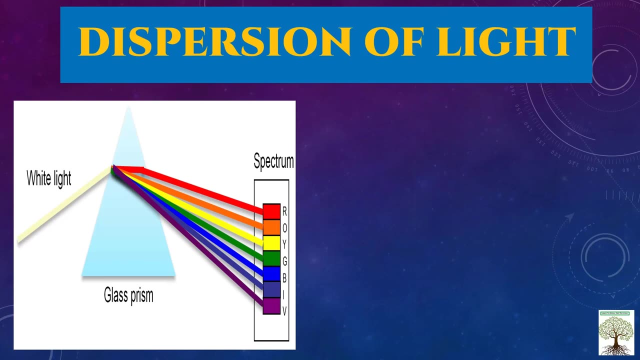 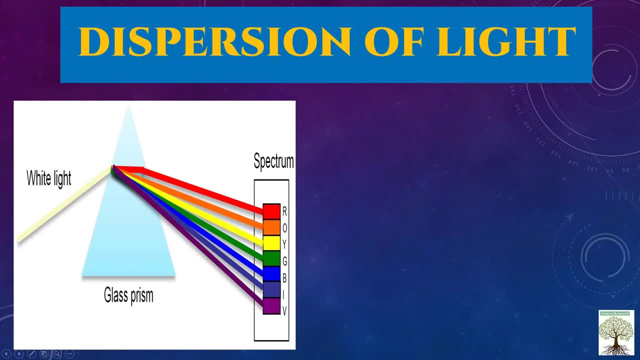 colors. so visible light can be split into seven colors. that is Vibhagore. you know that violet, indigo, blue, green, yellow, orange and red color. so visible light can be split into seven colors. the formation of rainbow also takes place due to splitting of light. see raindrops scatter sunlight into. 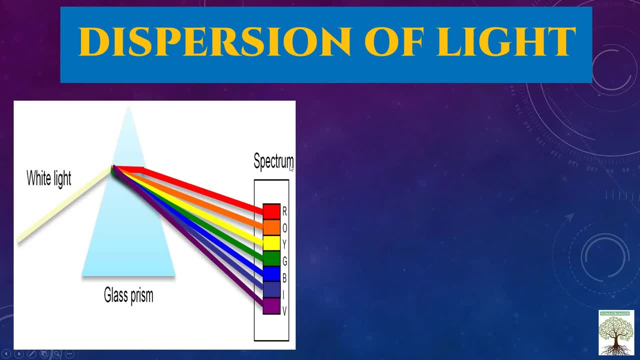 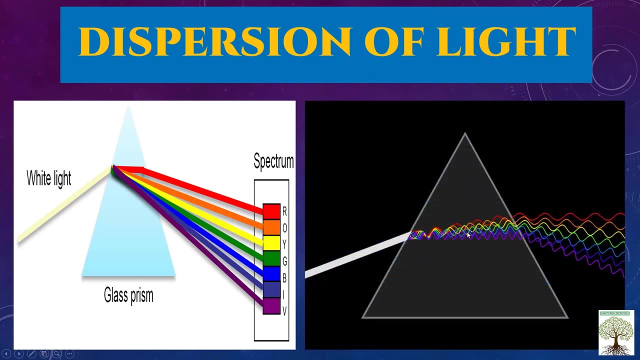 its seven colors to form a rainbow. so this is known as dispersion of light. when light pass through the prism, it will disperse into seven colors. ok, Vibhagore, this is the dispersion of light. property of light: see this? ok, white light. always. it is made up of seven colors, which are represented as 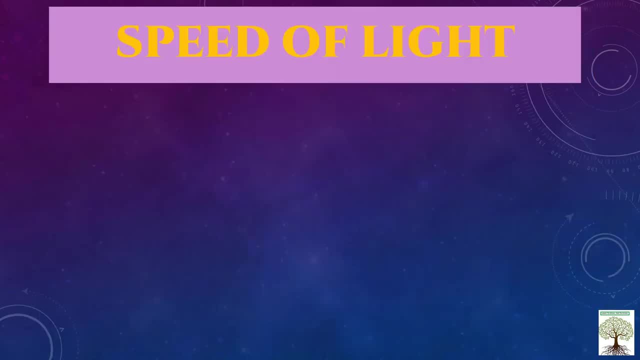 Vibhagore: speed of light. what is the speed of light? this is the next property of light, that is, the speed of light is 3 x 10 is to 8 meter per second. that means that is 2,99,792 kilometers per second. can you imagine the speed of light here? 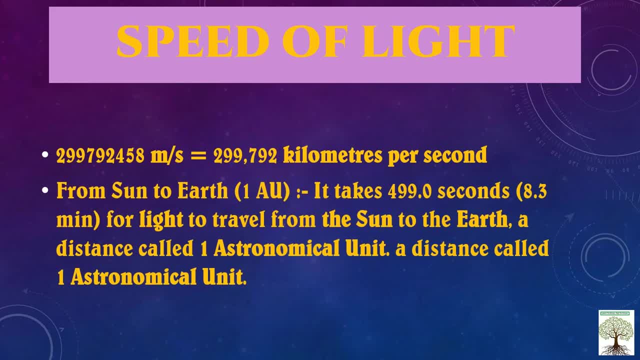 from Sun to earth- one astronomical unit that is known as from sun to earth. it takes 499 seconds only for light to travel from the sun to the earth, a distance called one astronomical unit. This distance from sun to earth is known as one AU. that is, one astronomical unit. It takes only 499 seconds. that means 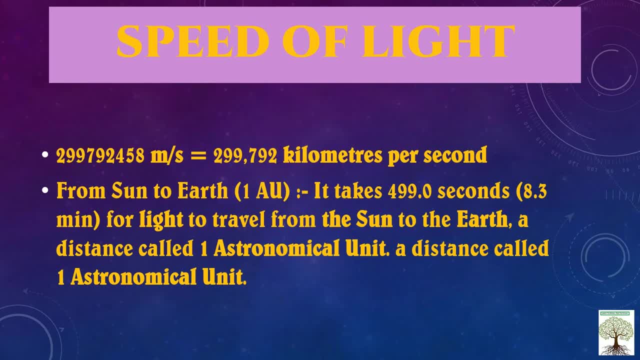 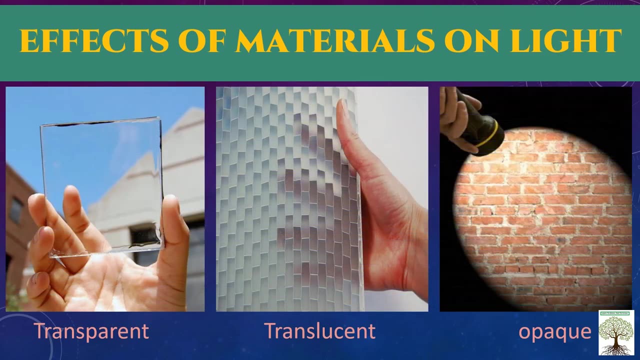 8.3 minutes for light to travel from the sun to the earth. This is the speed of light. 3 x 10 is 8 meter per second. Effects of materials on light. Can you see this? 3 materials First is transparent object. 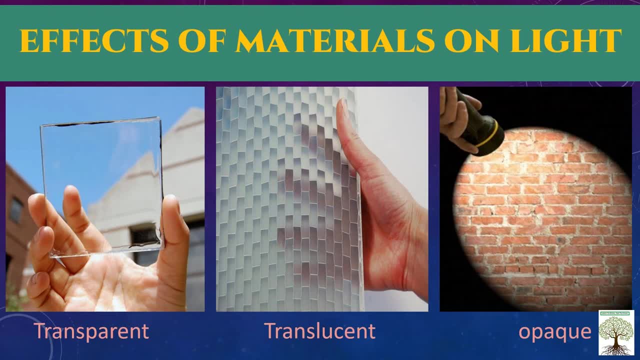 second: translucent. and the last one is opaque object, Transparent object. light can pass completely through these objects, like transparent objects, glass or clear water and air is also transparent object. So light can pass completely through these objects. transparent object. second kind of object: those 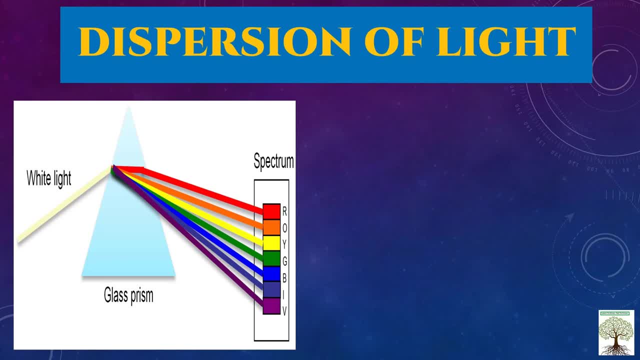 The formation of rainbow also takes place due to splitting of light. See: raindrops scatter sunlight into its seven colors to form a rainbow, So this is known as dispersion of light. When light passes through the prism, it will disperse into seven colors. 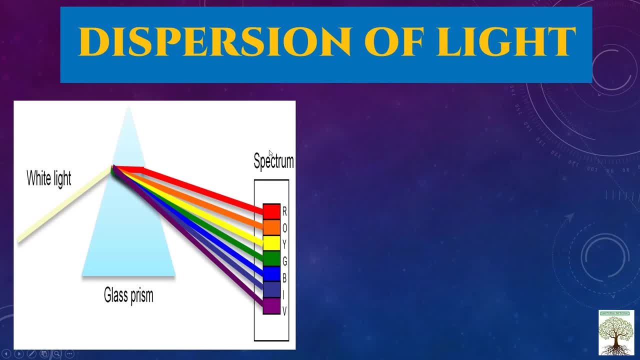 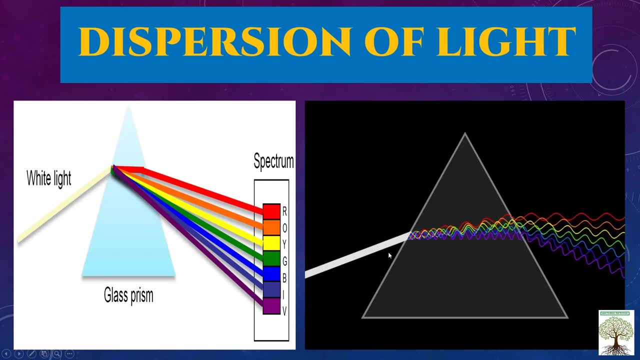 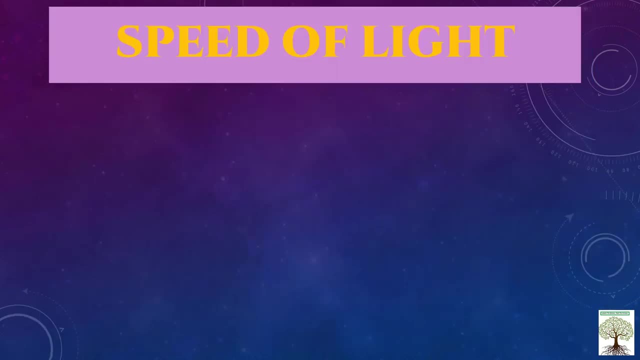 colors. ok, with your. this is the dispersion of light. property of light. see this, ok, white light, always. it is made up of seven colors which are represented, as with your, speed of light. what is the speed of light? this is the next property of light, that is, the speed of light is 3 x 10 is to 8 meter per second. that 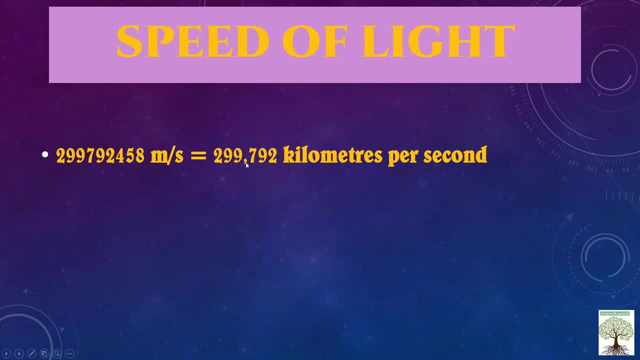 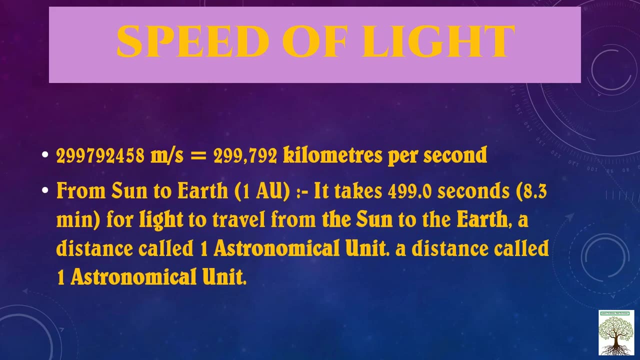 means that is 2 lakh 99,000 792 kilometers per second. can you imagine the speed of light here from Sun to Earth? 1 astronomical unit that is known as from Sun to Earth. it takes 499 seconds only for light to travel from the. 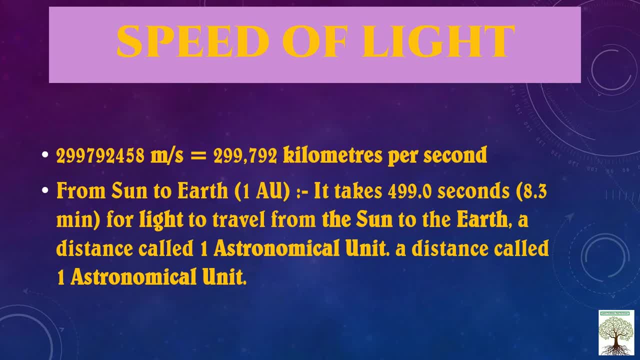 Sun to the Earth, a distance called 1 astronomical unit. this distance from Sun to Earth is known as 1 au 3. that is, 1 astronomical unit. it takes only 499 seconds. that means 8.3 minute for light to travel from the Sun to the Earth. this is the speed of light 3 x 10. 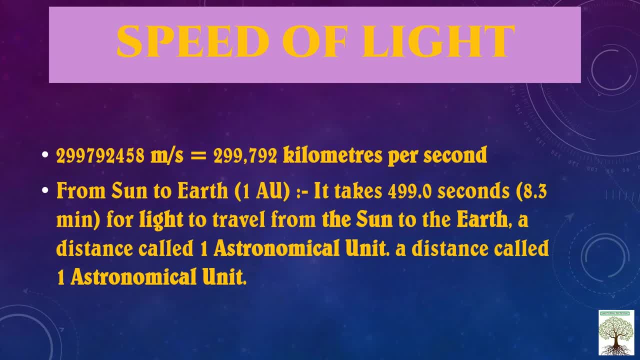 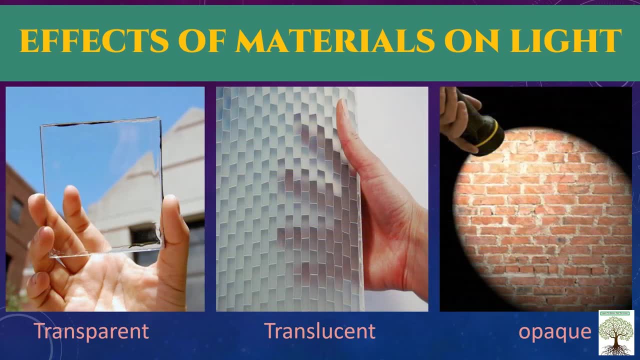 is to 8 meter per second. ok, effects of materials on light. can you see this? three materials: first is transparent object, second translucent and the last one is opaque object. transparent object: light can pass completely through these objects, like transparent objects- glass or clear water- and air is also transparent object, right, so light. 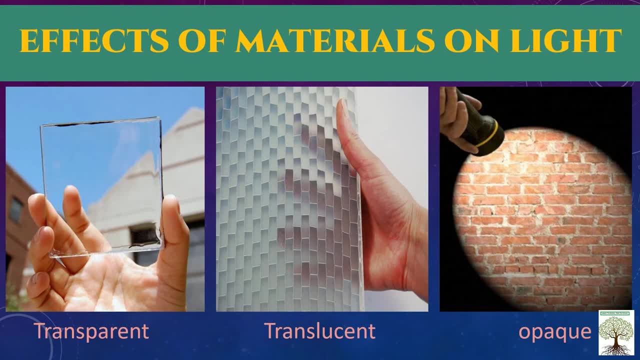 can pass completely through these objects. transparent object. second kind of object: those are translucent object like frosted glass or colored glass, butter, paper. these all are translucent object. only some light can pass through these objects so that objects seen through the translucent material appear blurred right. so because some light can pass through these type of object, translucent. 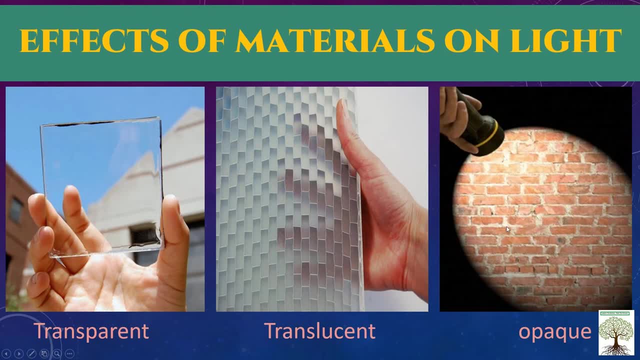 object. the third type of object objects are opaque object. light cannot pass through these objects because objects that completely block light from passing through them are known as opaque object right. so they will not allow light to pass through them because they block light completely, so that lights cannot. 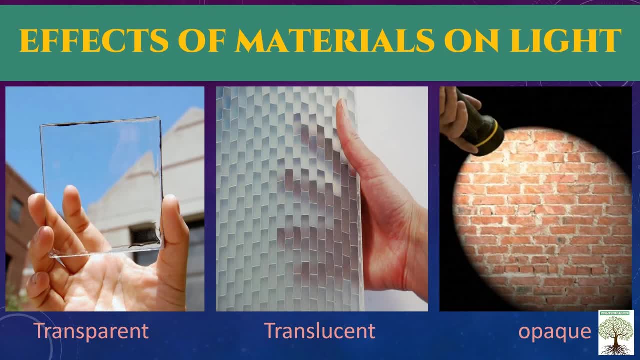 pass through these type of object. we cannot see anything through an opaque object like a wooden plank or table chair, wall, steel plate, right, these all are examples of opaque objects. so this is the property of light. light can completely pass through the transparent. some light can pass through the 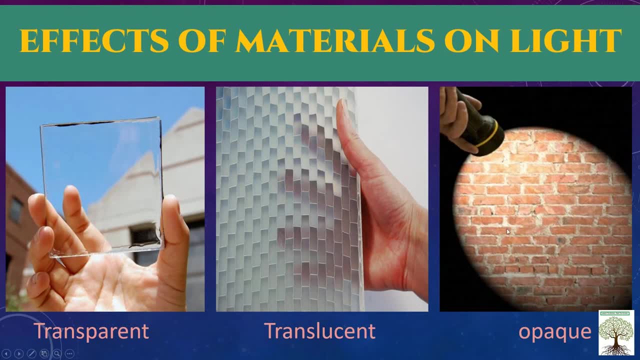 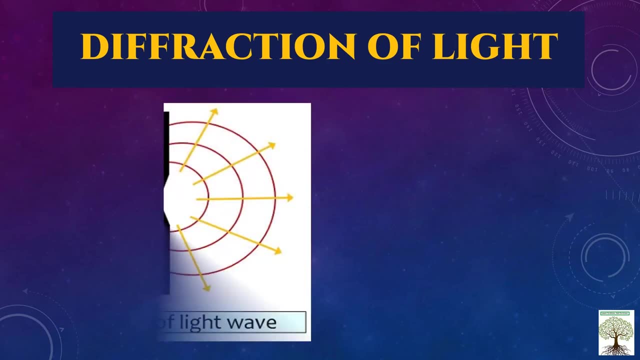 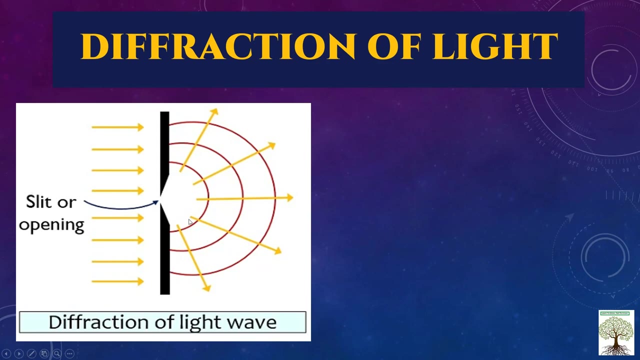 translucent and no light can pass through the opaque object. this is the property of light. next property is diffraction of light. what is diffraction of light? as you can see here, that is, the slit or one opening hole is there. so when light pass through this hole, it will defect it in the different 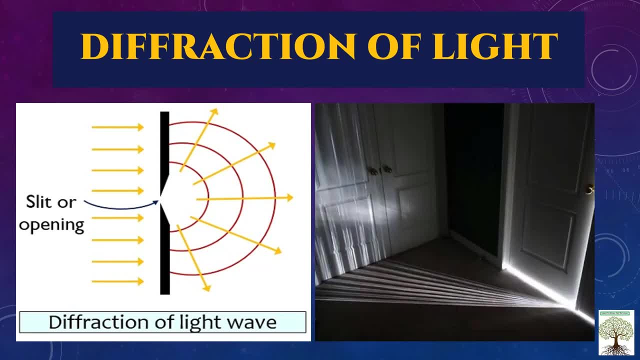 direction. so we can say that diffraction is defined as the spreading out of the wave as it passes through a small opening, a. So diffraction is the spreading of waves that happens when it passes through a narrow opening or when it passes around a small obstacle along its path. 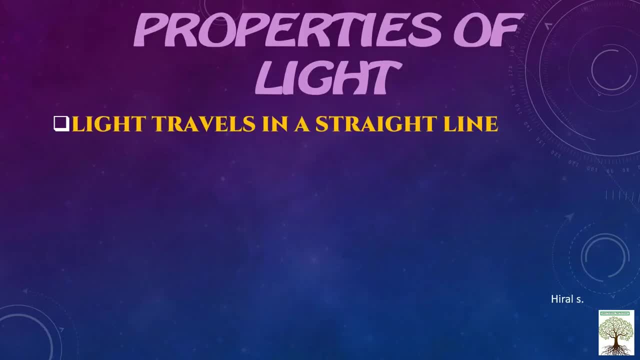 This is the property of light. diffraction of light. So these all are the properties of light. Light travels in a straight line. Reflection of light or bounce back the light. Diffraction of the light. Bending of the light at the boundary of the different medium. 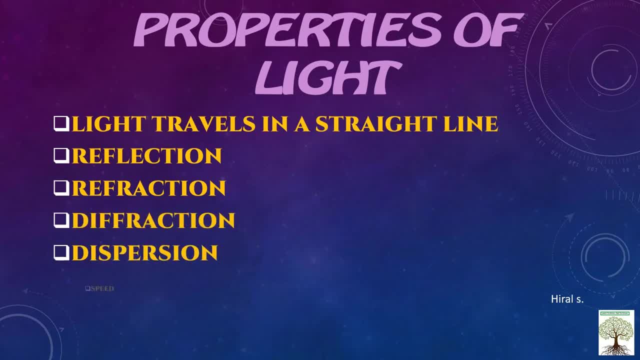 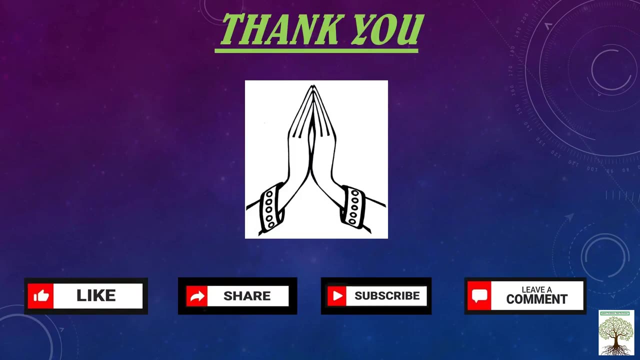 Then diffraction of the light, Dispersion of the light, Speed of light And effects of materials on light like transparent, translucent and opaque object. Okay, I hope these properties of light understood nicely, children. Thank you Like, share and subscribe my channel. 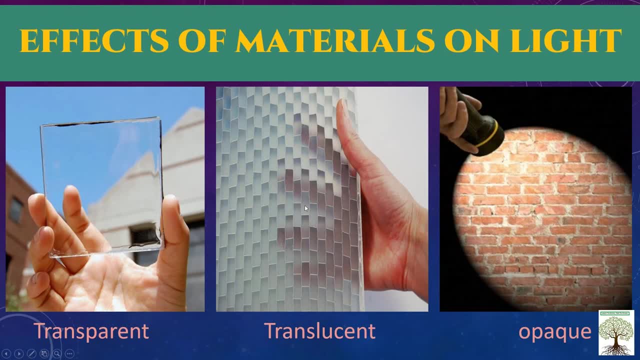 are translucent object, like frosted glass or colored glass, butter paper. these all are translucent object. only some light can pass through these objects, so that objects seen through the translucent material appear blurred right. so because some light can pass through this type of object. translucent object. the third type of object: objects are opaque object. light cannot. 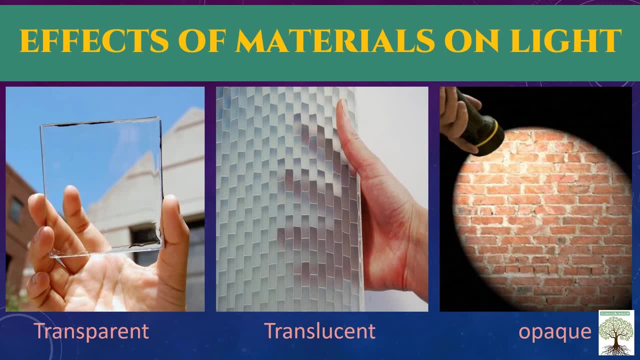 pass through these objects, because objects that completely block light from passing through them are known as opaque object right, so they will not allow light to pass through them, because they block light completely, so that lights cannot pass through this type of object. we cannot see anything through an object. 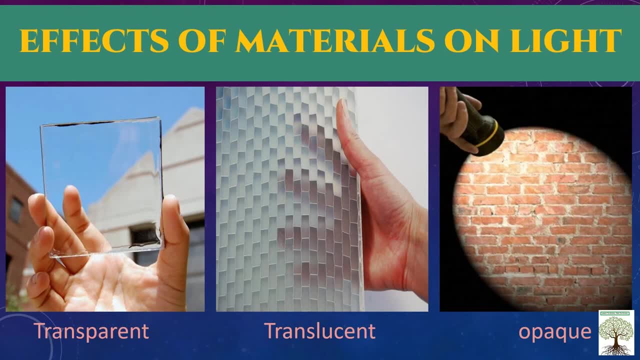 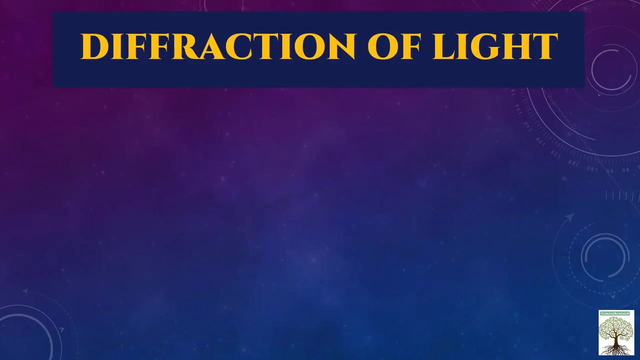 like a wooden plank or table chair, wall, steel plate right. these all are examples of opaque objects. so this is the property of light. light can completely pass through the transparent, some light can pass through the translucent and no light can pass through the opaque object. this is the property of light. next property is diffraction of light. what is diffraction of light? as you can, 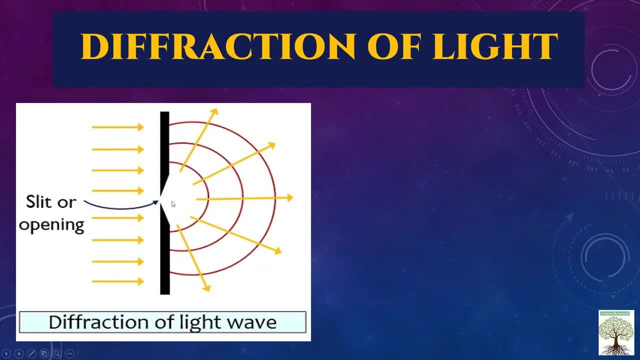 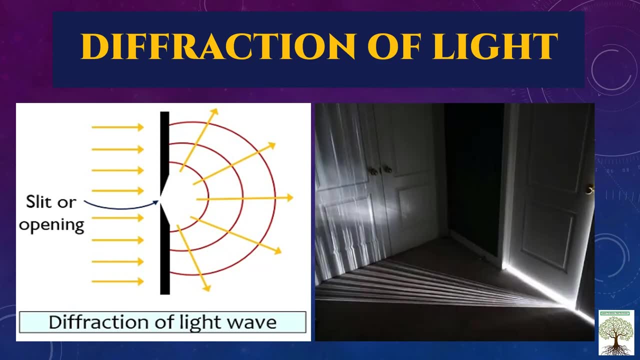 see here. so there is a slit or one opening hole is there. so when light pass through this hole, it will diffract it in the diffract it in the different direction. so we can say that diffraction is defined as the spreading out of the wave as it passes through a small opening. 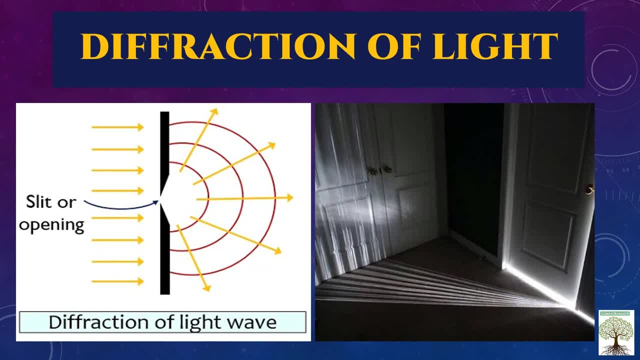 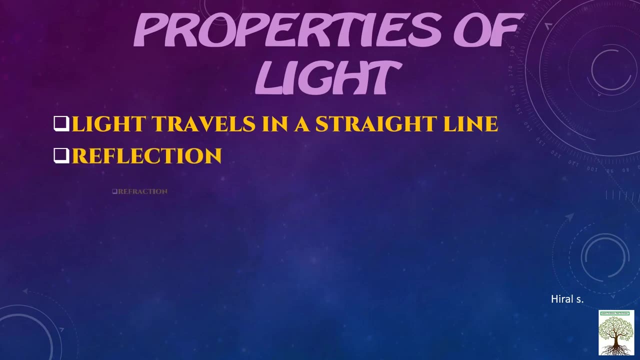 so diffraction is the spreading of waves. that happens when it passes through a narrow opening or when it passes around a small obstacle along its path. this is the property of light. diffraction of light. so these all are the properties of light. light travels in a straight line reflection. 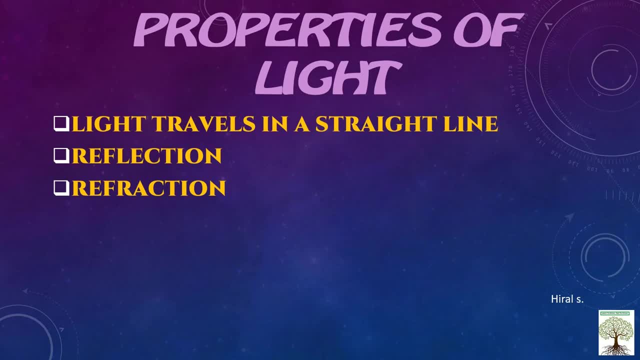 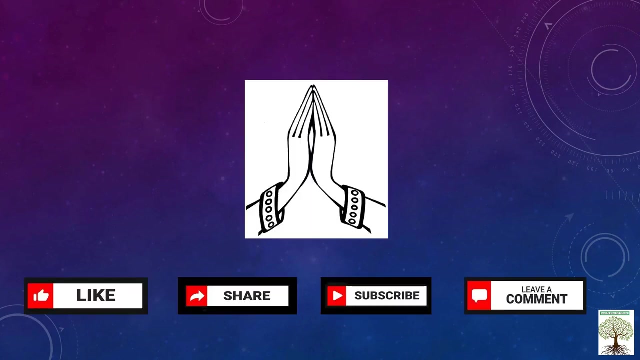 of light or bounce back the light. diffraction of the light, bending of the light at the boundary of the different medium, then diffraction of the light, dispersion of the light, speed of light and effects of materials on light like transparent, translucent and opaque object. okay, i hope this properties of light understood nicely children. thank you like, share and subscribe. my channel. learn to grow, not to know.